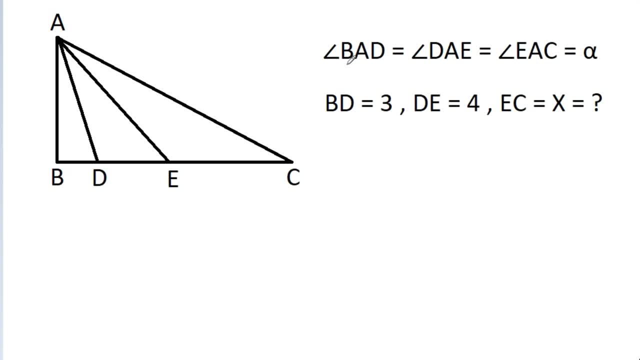 In this video we have given that Angan BAD is equal to Angan, DAE is equal to Angan. ESC is equal to ANFA. So Angan BAD is ANFA, Angan DAE is ANFA and Angan ESC is ANFA. 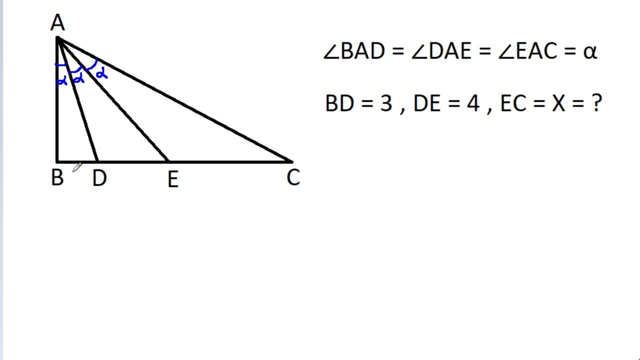 And BD is equal to 3.. This is 3.. And DE is equal to 4.. It is 4.. And EC is equal to X. It is X And we have to find the value of X. So the first method. 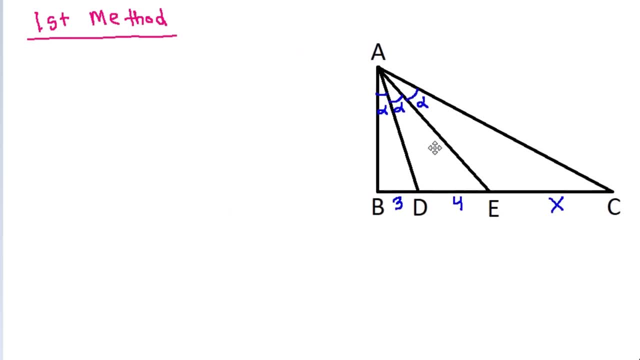 This is the figure And in triangle A, B, E, AD is Angan bisector And in any triangle A, B, C, if AD is Angan bisector, that means if this Angan is theta and this Angan is theta. 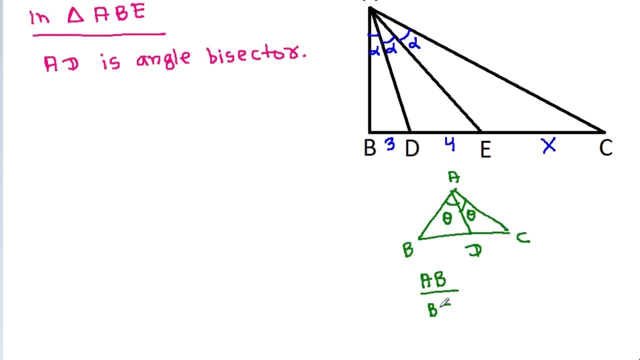 then AB by BD is equal to SC by DC. So in triangle A, B E, AD is equal to SC by DC. So in triangle A, B E, AB by BD will be equal to AE by DE, And it is: AB by AE is equal to BD by DE. 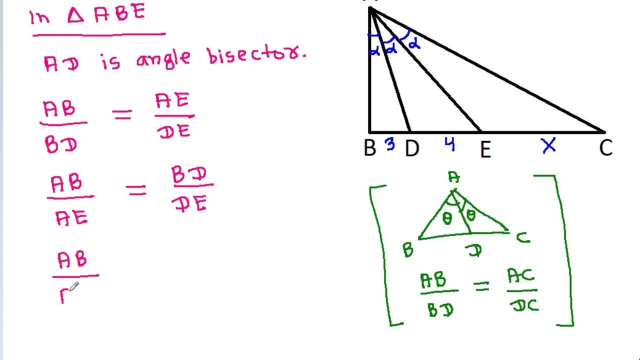 And AB by AE is equal to BD by DE And Então, if AB is equal to BD, is equal to 3 times some K, then AE will be equal to 4K. That means, if AB is equal to 3 times some K, then AE will be equal to 4K. 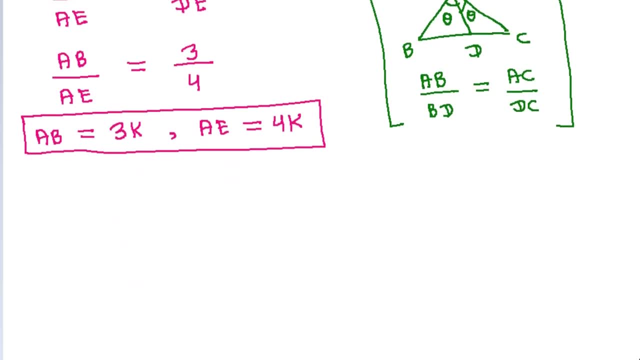 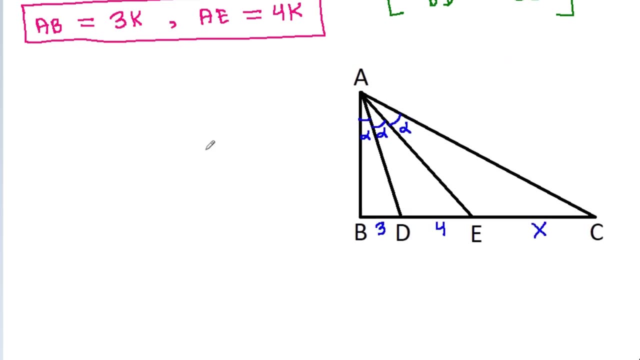 And, And, And, And, And, Then, Then, Then, Then, Then Again. inter angle ABE. this angle is 90 degree. That means AB square plus BE square will be equal to AE square by Pythagoras theorem, And AB is 3k squared. 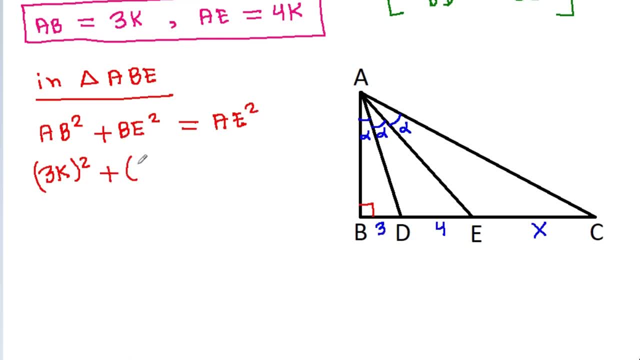 plus BE is 3 plus 4.. it is 3 plus 4. square is equal to AE is 4 k squared and 9 k squared plus 7. squared is 49 is equal to 16 k squared and 49 is equal to 50 k, and 50 ÷ 8 is equal to 50 k. 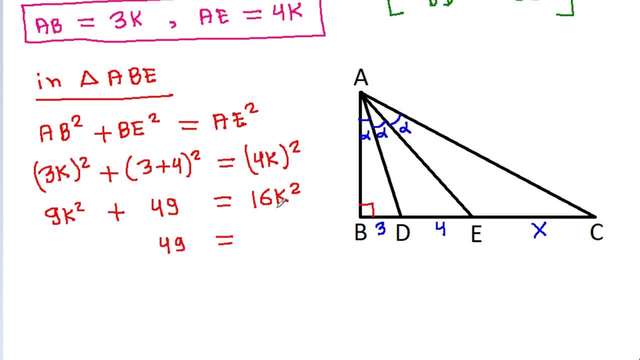 And 49 is equal tovadrender power, So our total volume of the Uzmanian is 11 kg. So our total volume of the Uzmanian is 11 kg will be equal to 16k square minus 9k square will be 7k square, So k square is equal to. 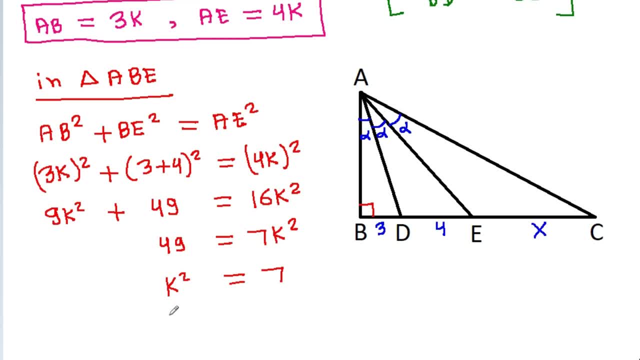 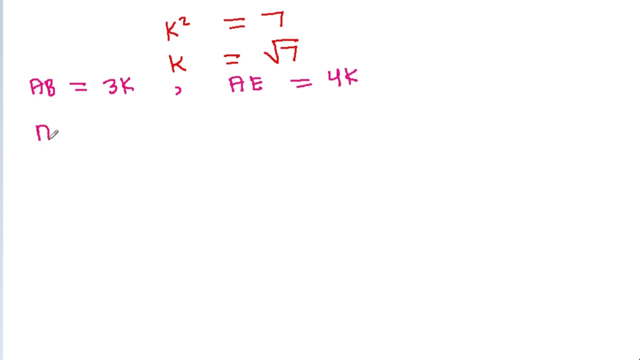 49 by 7 is 7 and k is equal to a square root of 7, because k cannot be negative And we have: ab is equal to 3k and Ae is equal to 4k. So ab will be equal to 3 root, 7 and Ae. 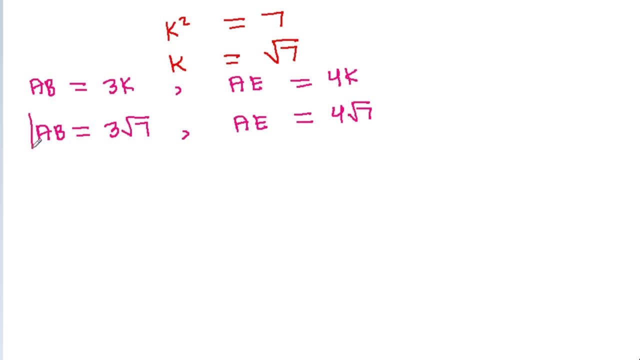 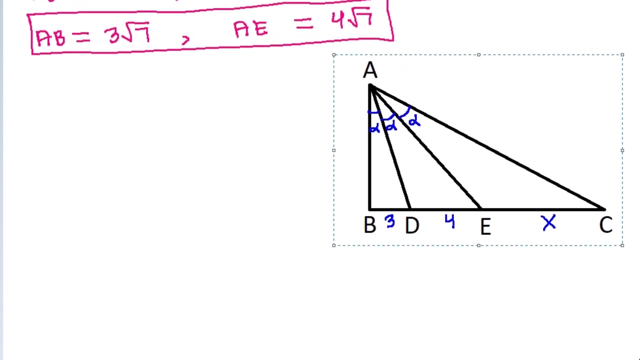 will be equal to 4 root 7.. And Now in triangle ABC, tan 3 alpha will be equal to BC by AB, and BC is 3 plus 4 plus X by AB is 3 root 7, and it is 7 plus X by 3 root 7. and in triangle ABE, tan alpha plus alpha. 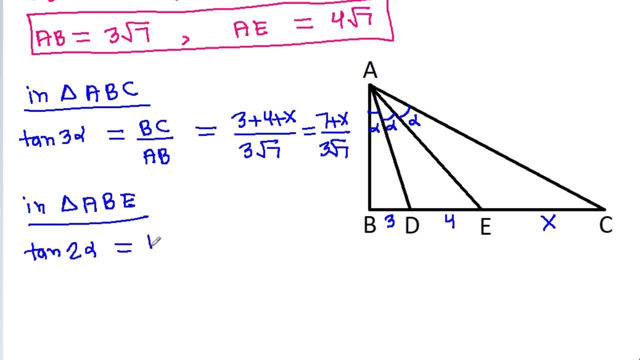 2 alpha will be equal to BE by AB and BE is 3 plus 4 by AB. Thank you, AB is 3 root 7 and it is 7 by 3 root 7, and in triangle, ABD tan alpha will be: 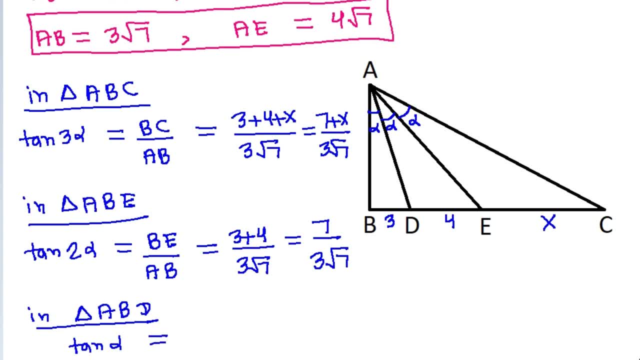 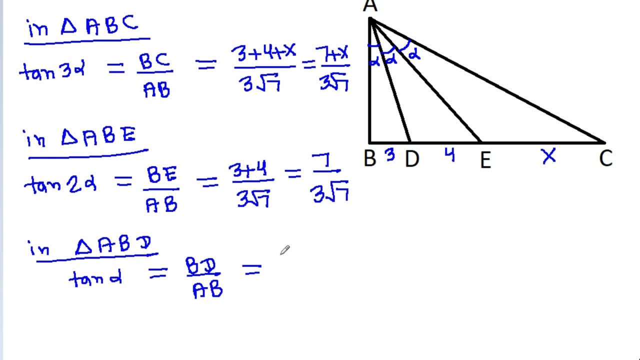 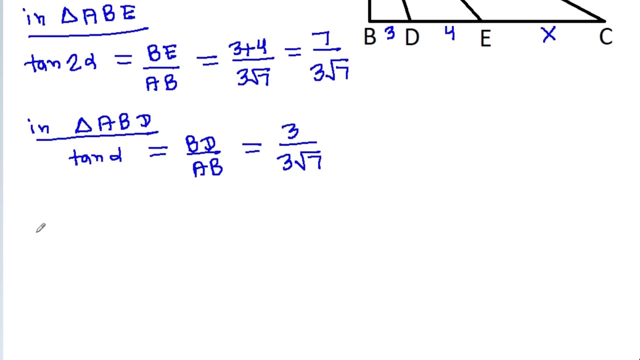 equal to BD by AB. It is BD by AB and BD is 3 by AB is 3 root 7, and we know that tanL alpha is equal to tan 2 antha plus antha, and tan a plus b is equal to tan a plus tan b by 1 minus tan a tan b. 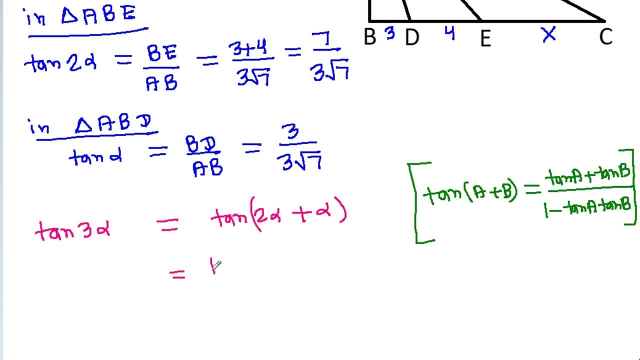 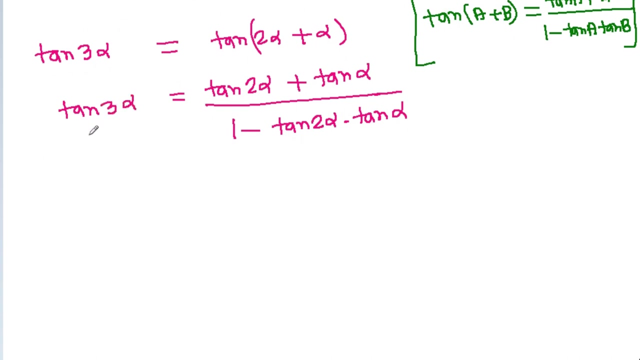 So tan 2 antha plus antha will be tan 2 antha plus tan antha by 1, minus tan 2 antha times tan antha, and it is tan 3 antha And tan 3 antha is 7 plus x by 3.. 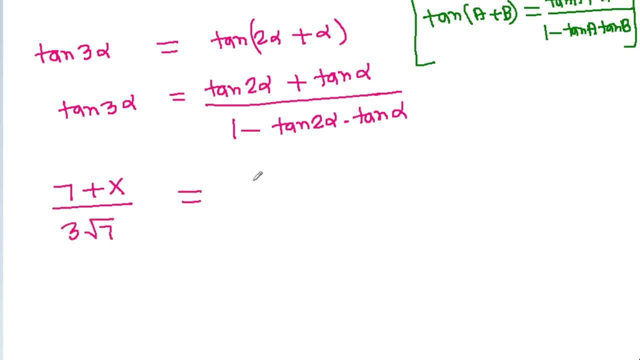 3 root 7 is equal to tan. 2 antha is 7 by 3 root 7. plus tan antha is 3 by 3 root 7 by 1. minus tan 2 antha is 7 by 3 root 7 times tan antha is 3 by 3 root 7.. 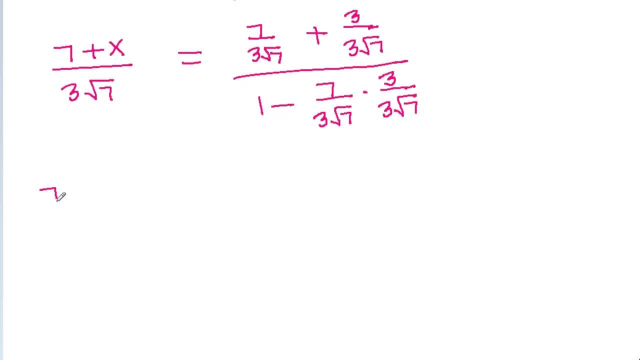 And It is 7 plus x by 3 root 7 is equal to: and this is 7 plus 3 by 3 root 7 by, and this is 3 root 7 times 3 root, 7 minus 7 times 3 by 3 root, 7 times 3 root 7.. 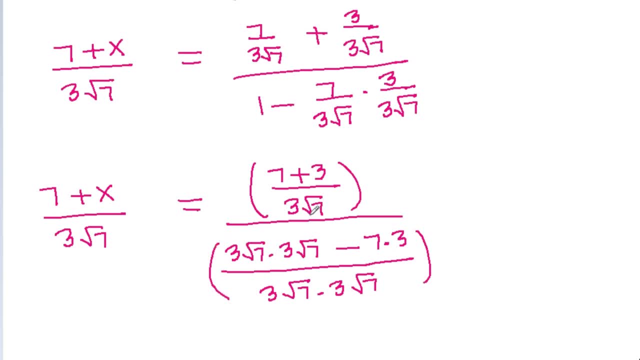 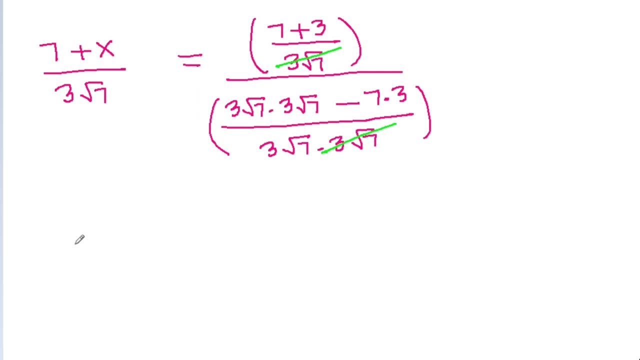 And 1, 3 root 7 will get canceled and it is 7 plus x by 3 root 7 is equal to 7 plus 3 times this 3 root. 7 by 3 root 7 times 3 root 7 minus 7 times tan x is equal to: 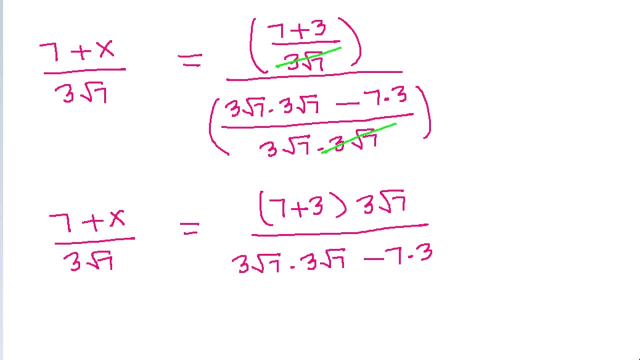 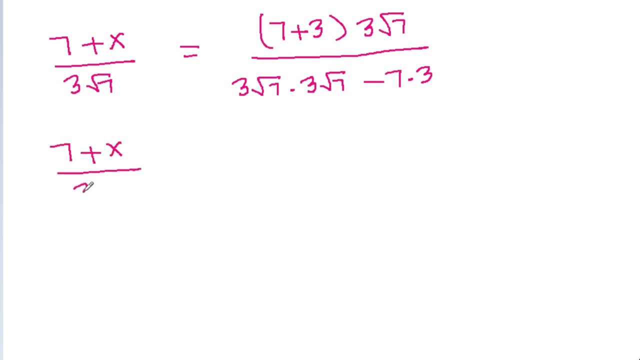 3 and it is 7 plus x. by 3 root 7 is equal to 7 plus 3 is 10 times 3 root. 7 by 3 root, 7 times 3 root, 7 will be 9 times 7. that is, 63 minus 7 times 3 is 21 and 7 plus x is equal to. 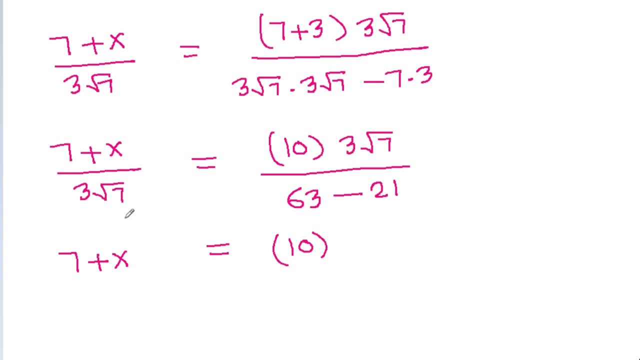 10 times 3 root. 7 times 3 root, 7 will be 63. by 63 minus 21 is 42, and 21 times 2 is 42 and 21 times 3 is 63. so 7 plus x is equal to 30 by 2 and 7 plus x is equal to 15. that means x is. 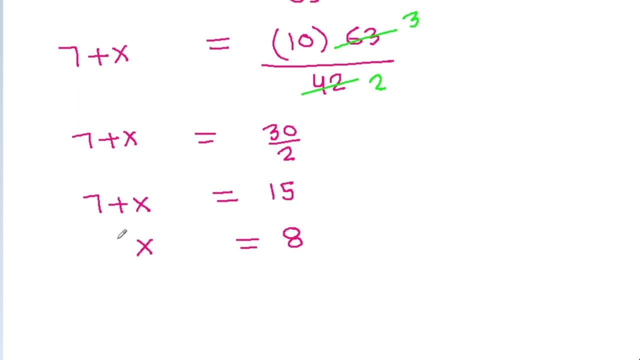 equal to 15 minus 7 is 8. and this second method is: this is the figure. and if we extend bd to suppose m and dissonant is 3 and join m, then dissonant will be equal to dissonant and this angle will be alpha. 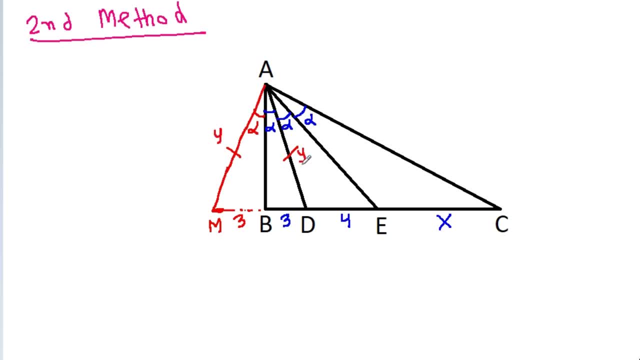 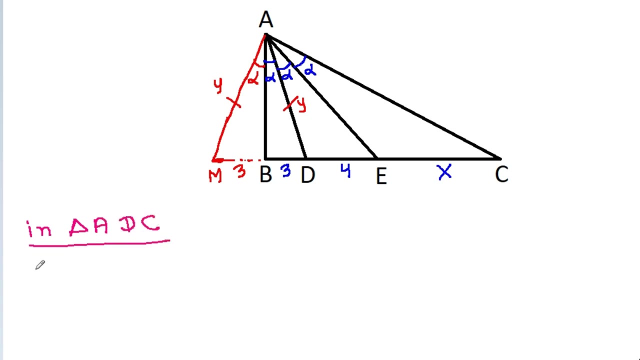 suppose dissonant is y. and now Ellis ADC. AE is angle bisector. that means AD by DE will be equal to AC by EC and inter angle AMC AD is angle bisector because this angle is 2a and this angle is. 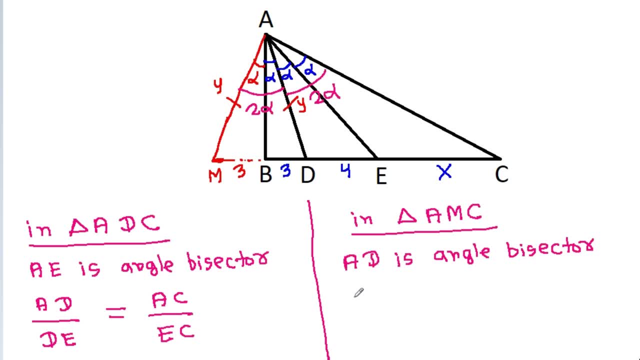 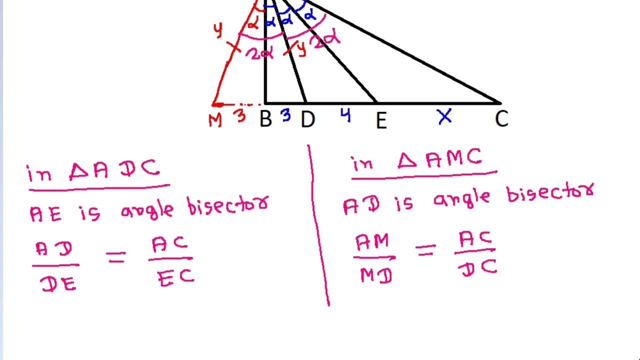 also 2a. That means AM by MD will be equal to AC by DC and AD is Y by DE is 4 is equal to AC by EC is 4.. That means AM by MD will be equal to AC by DC and AD is Y by DE is 4..